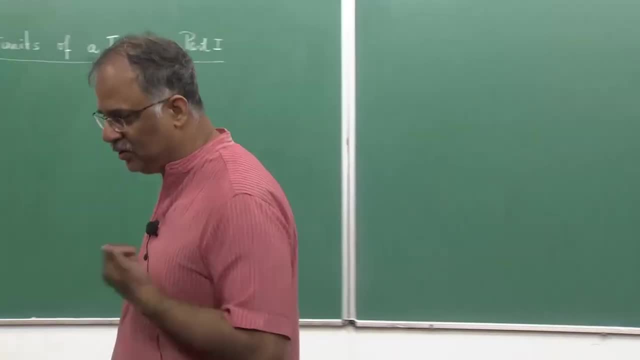 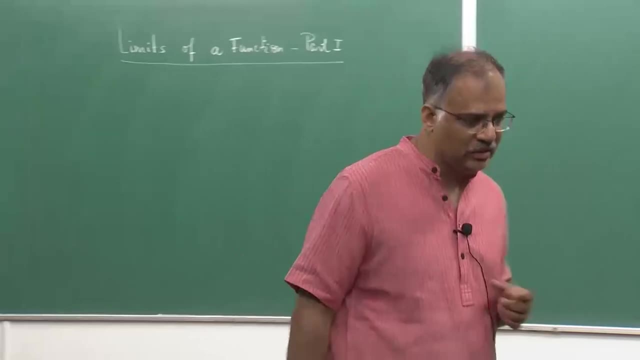 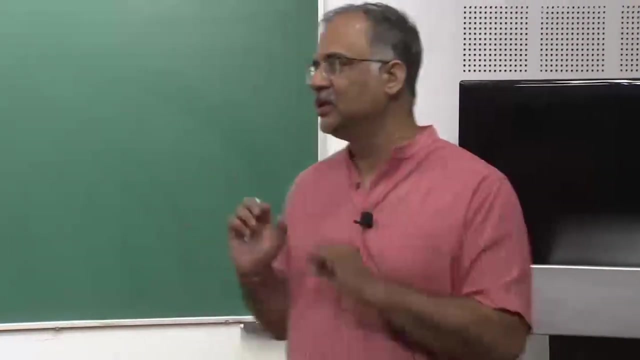 all those things. I would suggest that you would keep this in mind, that you would understand calculus for better if you know at the very outset that these derivatives and integrals are names given to some special kind of limits. So limit is actually the most central and 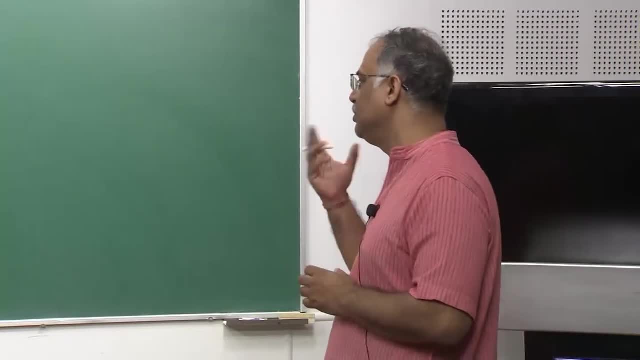 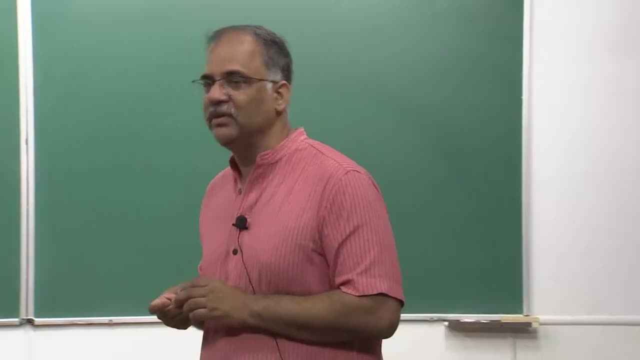 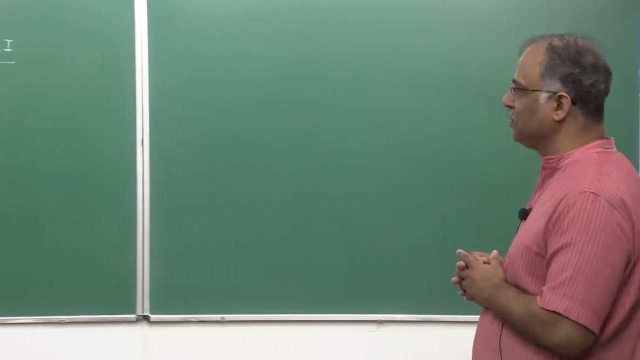 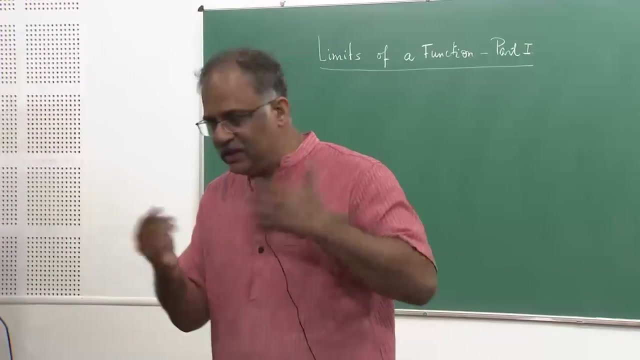 possibly sometimes viewed as a very slightly difficult concept in calculus. and you will understand calculus much better if you know at the very outset that every continuous function did not have a derivative. We will come to all those things later, but first of all let me tell you what is calculus actually. What does calculus study? It is just to, is it just? 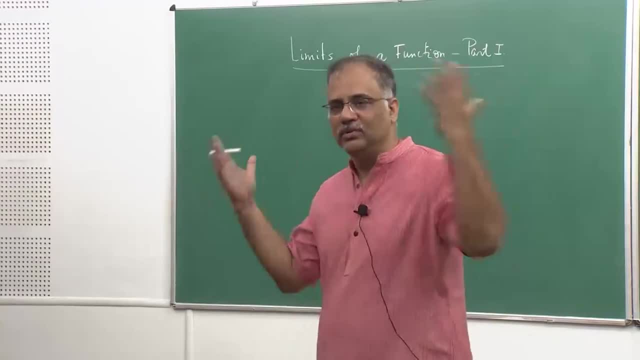 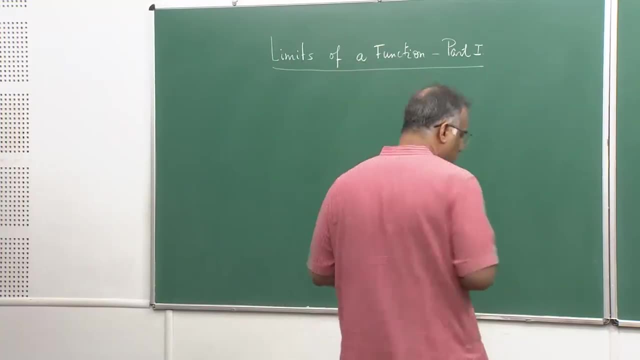 to write some derivatives, something from the air, and then you just get some marks in the exam. So what is calculus examination? Is that for the reason for which you study calculus? Of course many of you would say I have to do it in my IIT, JEE, I have to give my engineering 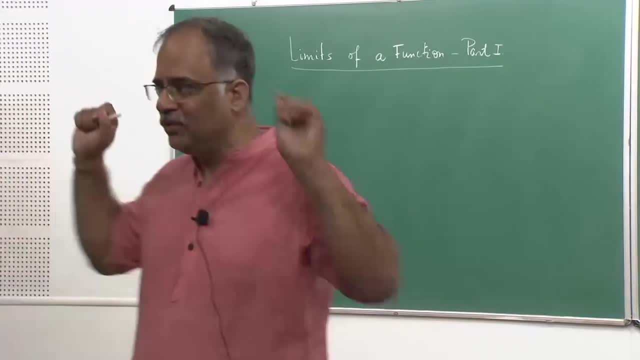 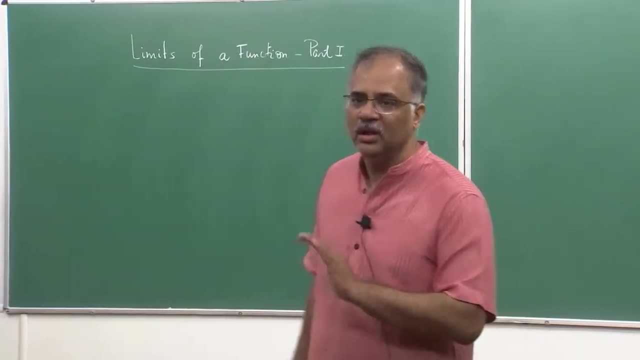 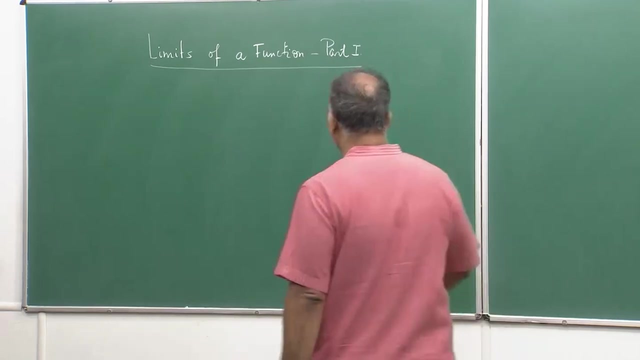 exam, math one course. So I will just do something. I have to know the tools I have to apply it. blah blah stuff. but the real issue, which is hardly seldom told in our class, is that calculus studies change. It tells you that if I have a function written in the form of 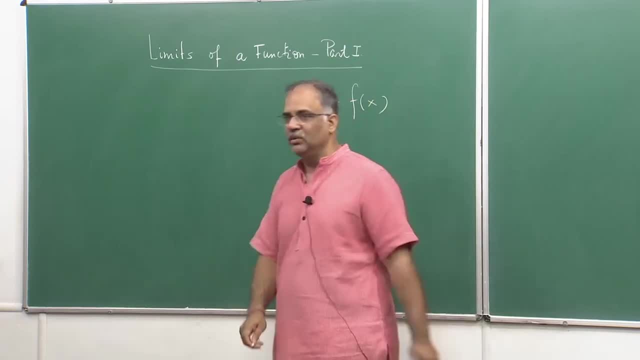 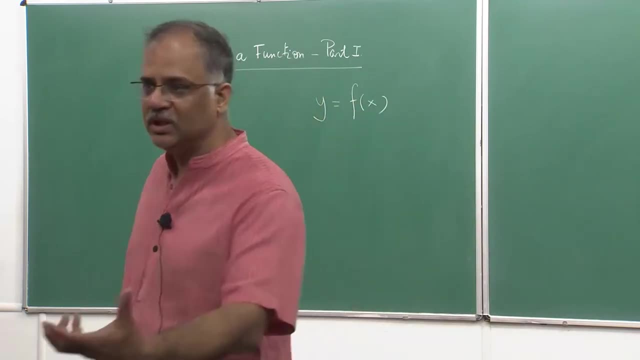 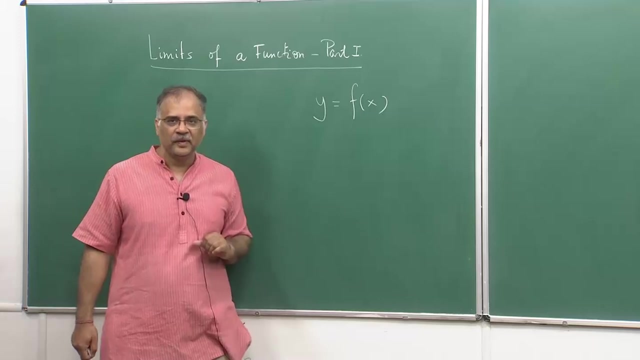 written in this form: y equal to f of x. then what happens to how? how does y changes when x changes? How does the function value change with the change of the independent variable, This x variable, which which we call the independent variable? and this is the dependent variable. 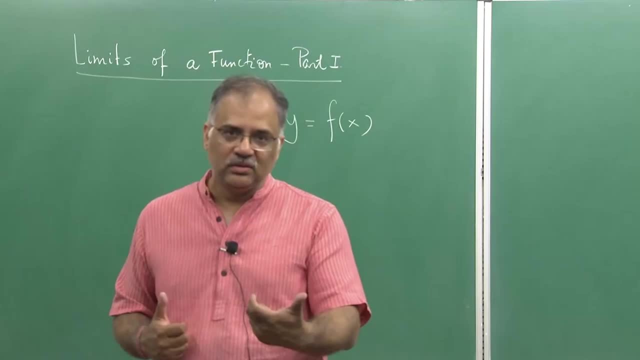 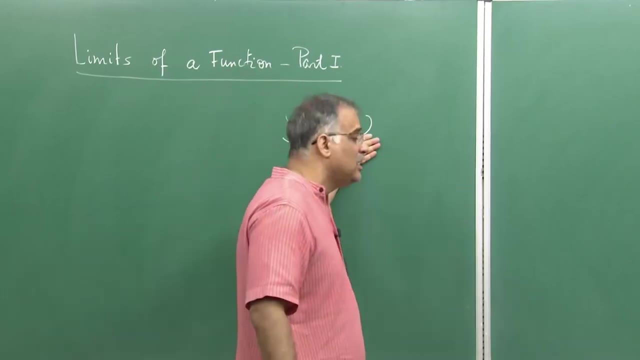 Calculus actually deals with the rate of change, change per unit time. So time also gets linked with calculus. This variable largely depends on the rate of change. The rate of change largely has been time talking about time. So calculus arose because people wanted to. 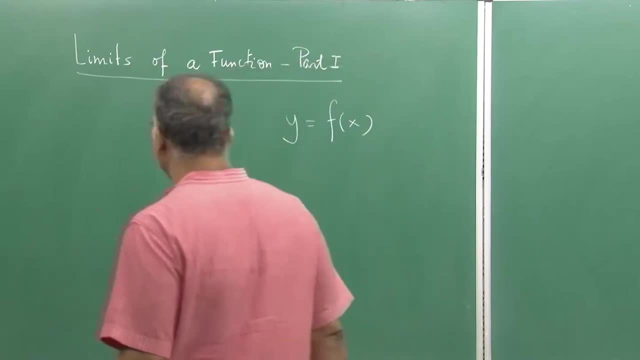 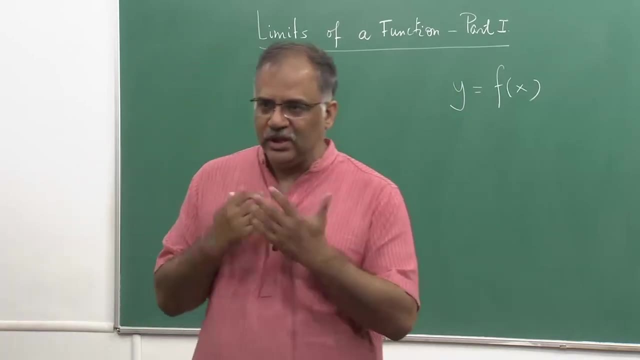 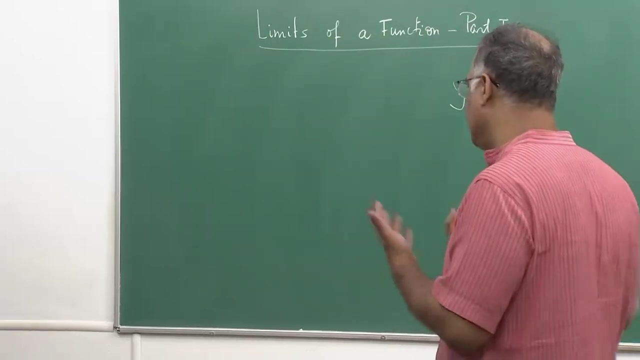 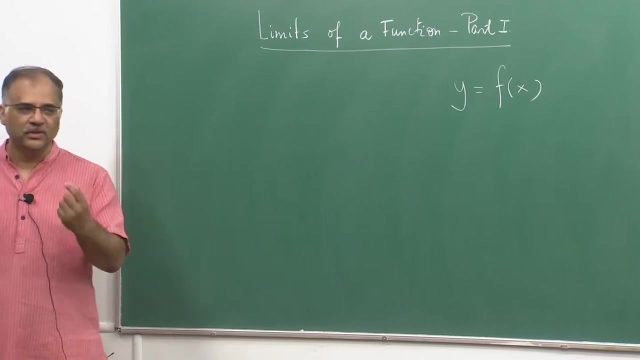 understand motion and if you read the or if you look at the history of calculus, it was essentially while trying to understand motion of bodies- motion of heavenly bodies rather- that calculus first took its root and it first came in when people started talking about the velocity of motion.